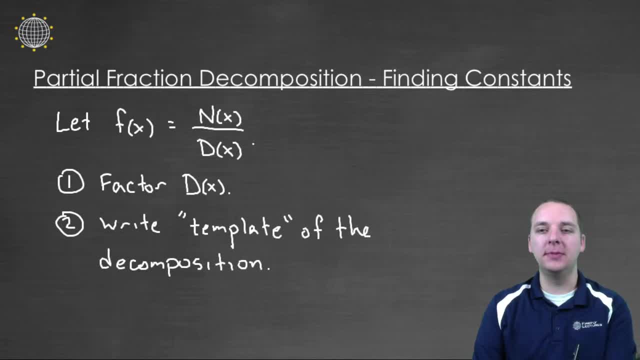 one that sort of thing. But we can write a template of the decomposition And then, when we're done, we can find the unknown constants in the numerator which will fill out or complete the template, Because initially when you write the template, you have something like A over. 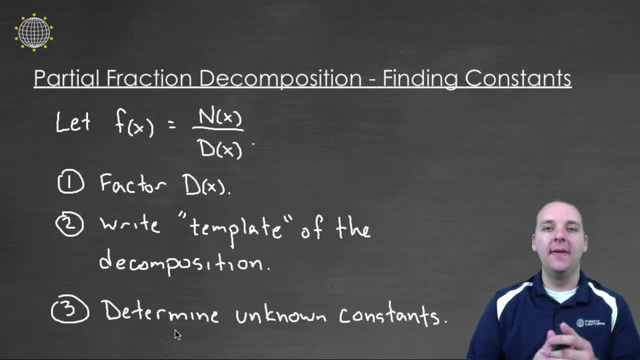 something plus B over something, plus C over something. And that's kind of the missing step. And in fact that's what we're going to talk about in this video. this last step: Finding these unknown A's and B's and C's, Finding the constants which are in your numerators. 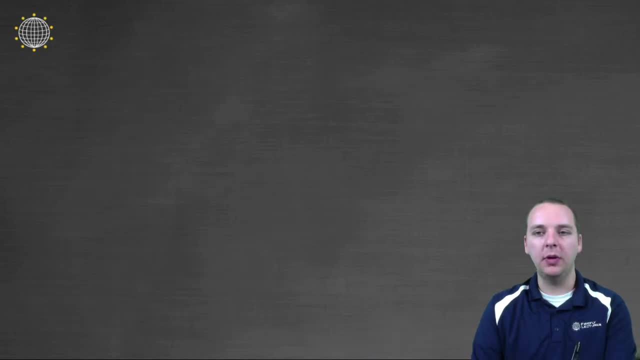 of your template for the decomposition. Okay, Alright, now there's two typical ways that are taught how to find. students are taught how to find these constants that are in the numerator. One way, one of the traditional ways, Is to use systems. right, There's a, there's a way, and, and we're not really going to- 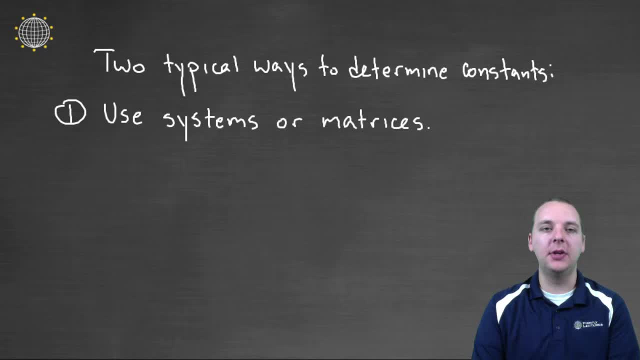 get into too much of these details for for this method in this video, But there's a way that you can construct a system where you have multiple equations with A's and B's and C's, etc. So, for instance, if you had an A and a B that were unknown, then you would get a. 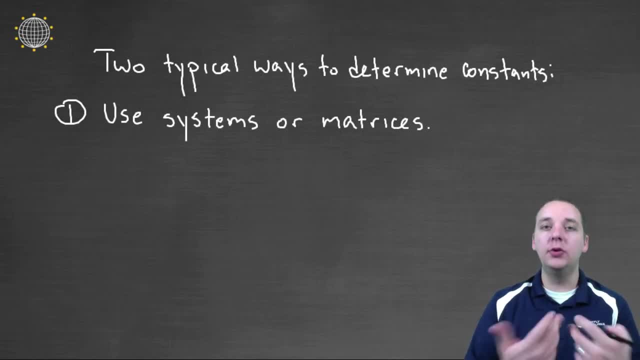 system of two variables or two unknowns and two equations And you could solve for the A or the B, And there's a way you can set up a system to do that, And that's what we're going to talk about in this video. 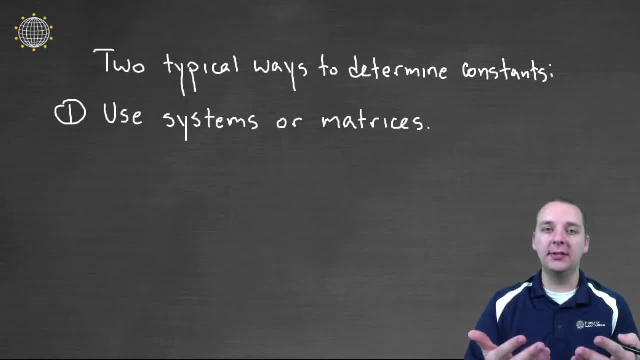 If you had an A and a B and a C, you could construct a system with three equations, with three unknowns, And it would allow you to solve for the A, the B and the C. This method is traditionally taught in like a college algebra class, Because it's usually taught. 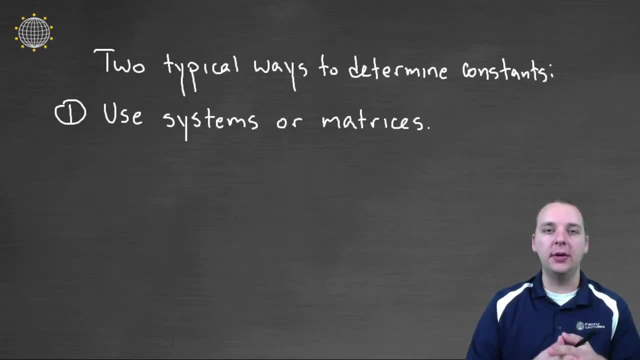 in the chapter on systems, And so it's a good practical use of systems. But if you're doing this in a calculus class, it's a little bit different. We don't really care too much about systems, We just want the answer. We just want to know what the A and the B and the 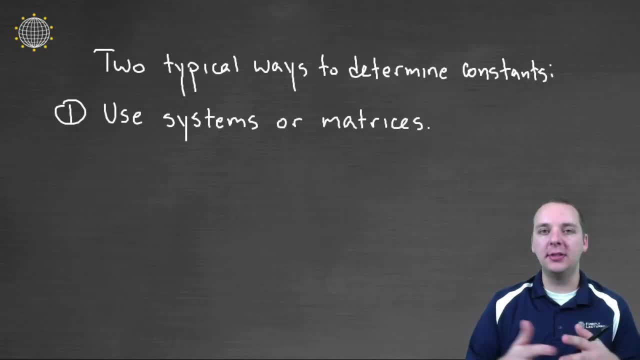 C are, And so we're going to think about that a little bit. So we're going to mention the first one we're going to talk about is the matrix, And the matrix is a function of the two collections that are in the system. So you can use a matrix to make a system And you can use a matrix. 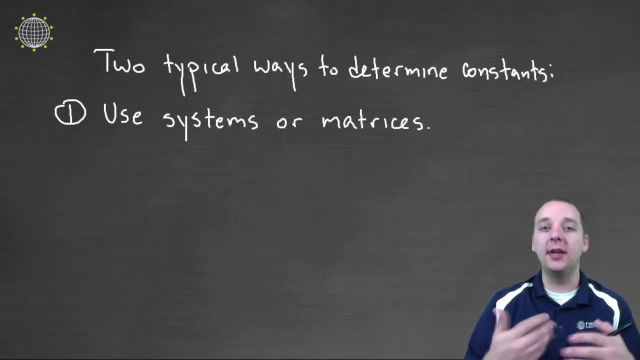 to make a system, So you could also use matrices, which ties together with systems. So it's a good technique to learn more about matrices as well. But usually in a calculus class like we're in, all that's all. that's a moot point. We don't. we don't really care too much about. 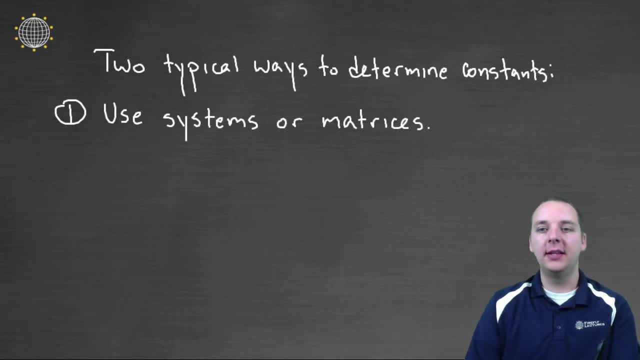 the systems. We just want to know what the A is, what the B is, what the C is, and let's be done with it. So it turns out there is also a shortcut. Now. you usually won't see this shortcut in your college algebra class. Sometimes I'll go ahead and teach it to the 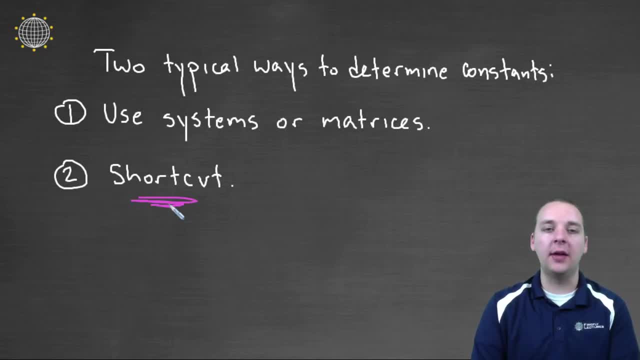 students anyway, just to kind of speed it up or allow them to check their work or that sort of thing. but it doesn't use systems and it's a little bit quicker. Rather than write out some formal steps, I think, I'll just show you how this shortcut works. Alright. so let's say we had an example. 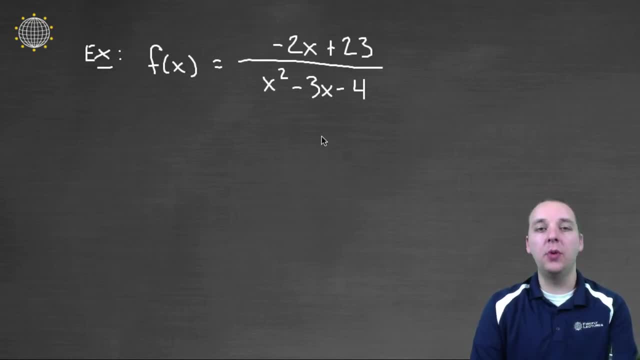 like this and we're trying to decompose it. So what will we do first? Well, I have n of x over d of x, and step one was to factor this denominator here. Okay, if you can, it's not always. 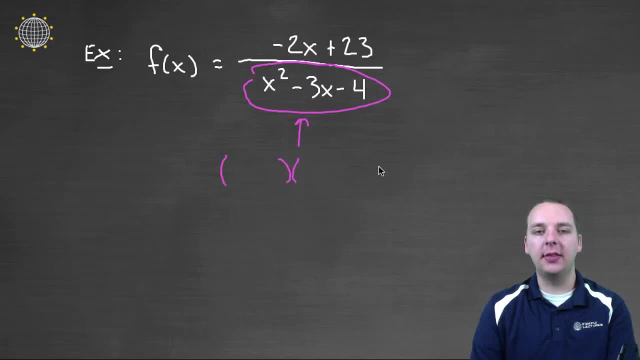 possible, but if we can. So let's see. does this guy factor? I think he does. It would be an x and an x, and it would be a minus four plus one, right, Minus four plus one, and so this would: 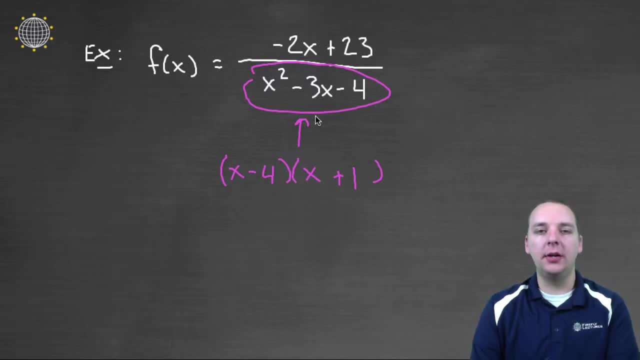 this would be the factored form of this denominator here. So what I'm going to do is I'm going to erase this. I'm going to put this in its place. Okay, so there we go. We have x minus four times x plus one, Excuse me. And the next step will be to write the decomposition. 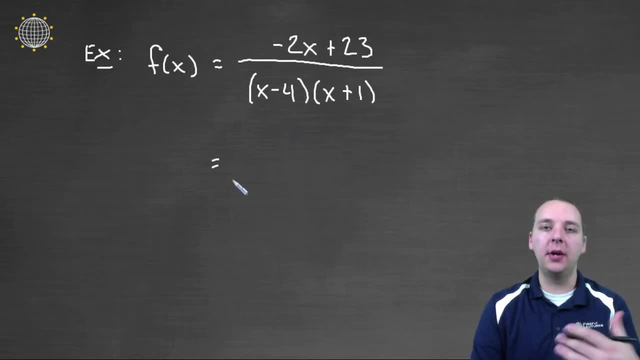 This is going to be the factored form of this denominator here, So what I'm going to do is I'm going to write the decomposition. This is that, that part that depends on what your denominator factors look like. Both of these are linear factors, So if you watch that video on how to 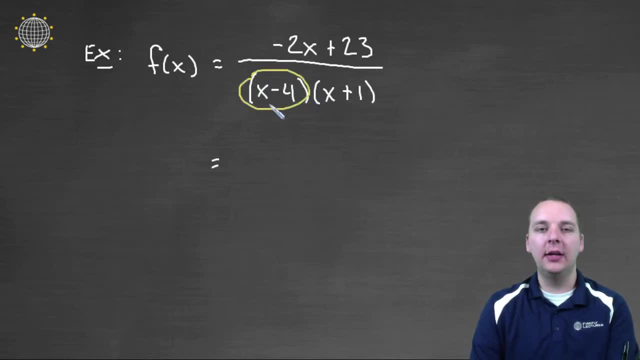 handle linear factors, then you would know that this guy contributes a term to the decomposition, namely a over x minus four, And this guy contributes one term to the decomposition: b over x plus one. Now, why did they only write the decomposition? Well, because they didn't. 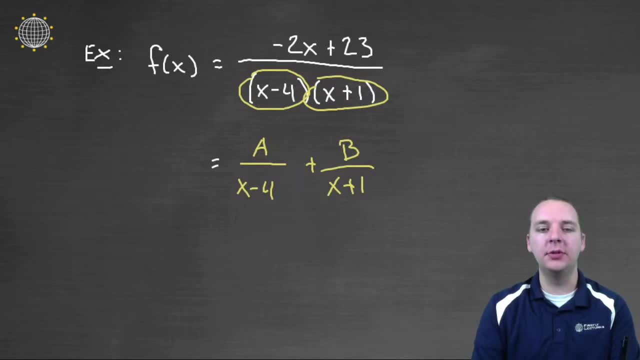 only contribute one term and not two terms or three terms individually. Well, that has to do with these powers. See, this is x minus four to the first power. This is x plus one to the first power. If this had been the second or third or fourth power, there would have been, you know. 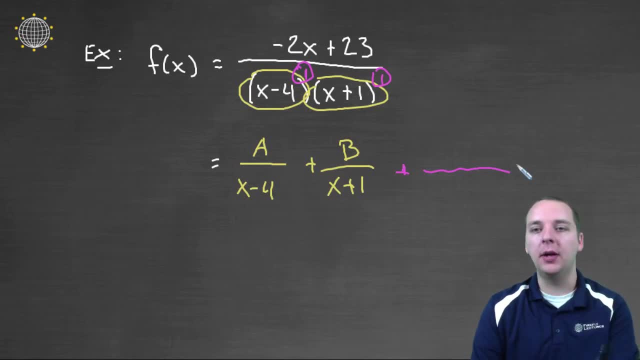 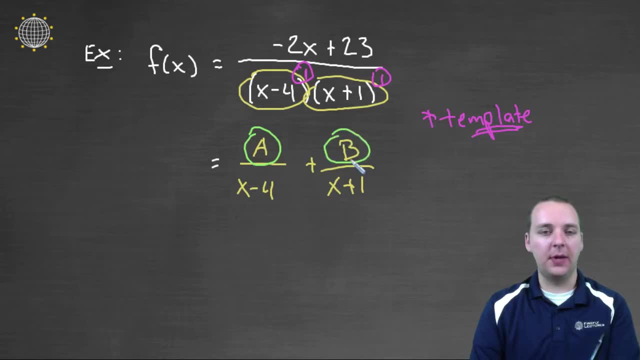 I have no idea what the a and the b are. I don't. I don't know what they are. All right, So that's what we're going to talk about: how to find. I'm going to show you a shortcut, Okay, So here's what. 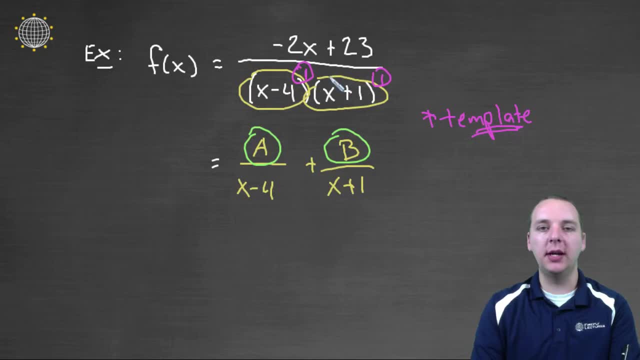 we're going to do. Let's, let's actually write this out as a as one straight line going straight across. I'll tell you what. I'll just do it on this card. I'll probably speed things up a little bit, rather than flip back and forth between the two different cards. Okay, So I'll tell you what. 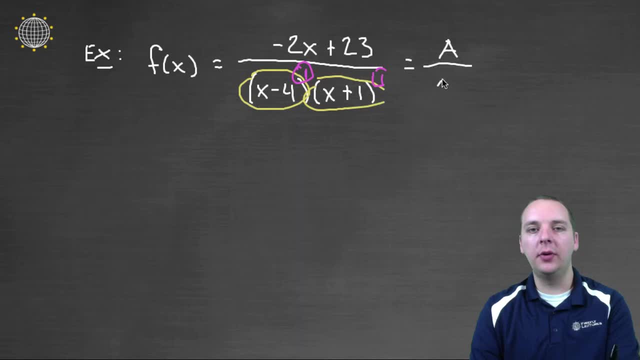 I'll just jot it up here in the corner real quick. We'd have a over x minus four plus b over x plus one. Okay, So the first step and you can make yourself little notes. I'm not going to write down all of these individual notes, but the first step is to get. 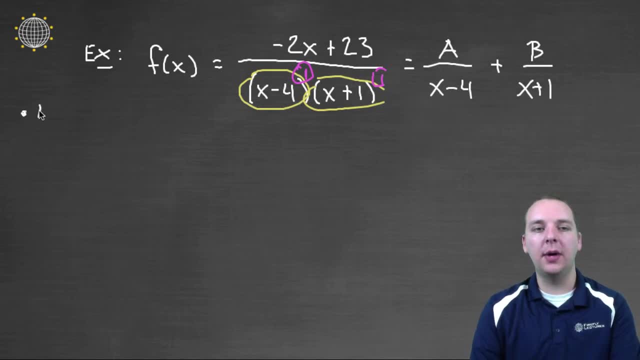 rid of the fractions by multiplying by the least common denominator- Probably familiar with the LCD from, like your algebra classes. but I need the lowest common denominator, or least common denominator between x minus four and b over x plus one. So I'm going to write down all of these. 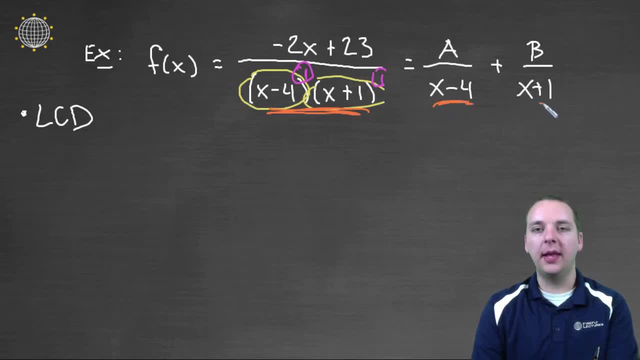 voltageيد for the list all together to get something easy: 2 or 3 times times x plus 1.. And this is zero. here's the picture. Okay, So all of this will be acting X minus 1.. Okay So. 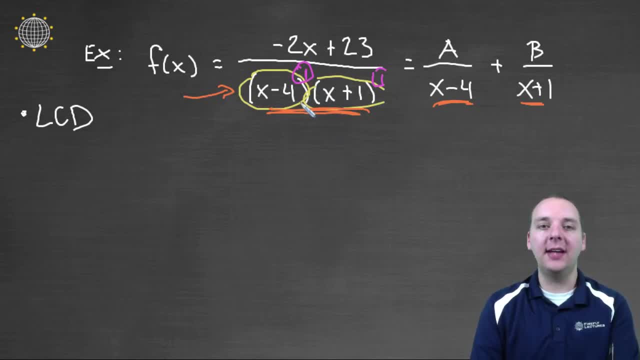 phrase: calculate it. Let's do that, And pretty good. Now, again, we're going to use the denominator from the left, cause the letter torx will be always – yeah, the letters that are floating in the left. So, whatever, the letter torx will be the denominator. You want to create an X facing. 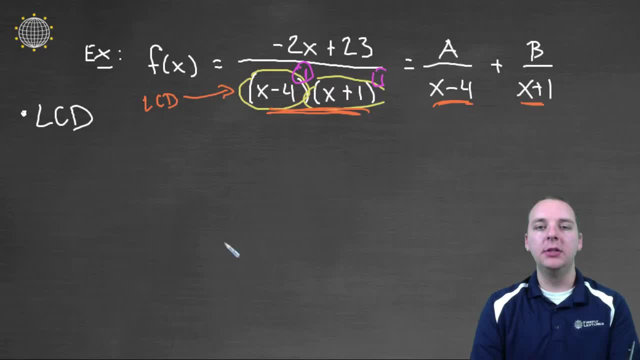 ten denominator will always be your LCD. So we're going to multiply that LCD through to both sides and that will get rid of our fraction. So let's do that. Multiply the left side by X minus four times X plus one. these cancel, cancel and you'll get negative two X plus. 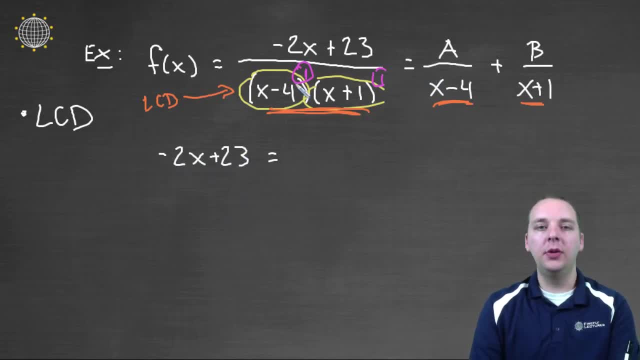 twenty-three, equal to. when you distribute the LCD to this term, the X minus fours cancel, but you still have an A and you still have an X plus one. When you distribute the LCD to this term, the B stays, the X plus ones cancel and you'll be left with an X minus. 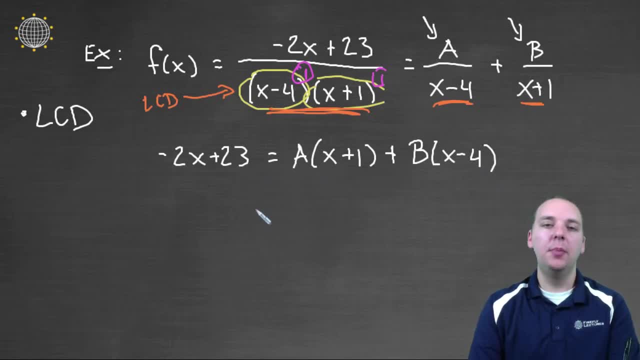 four this time. Alright, so we get this equation, but it's not an equation like you would traditionally think. This is not an equation that has right answers and wrong answers. This is, this is what's called an identity. This should always be equal to this, And here's the 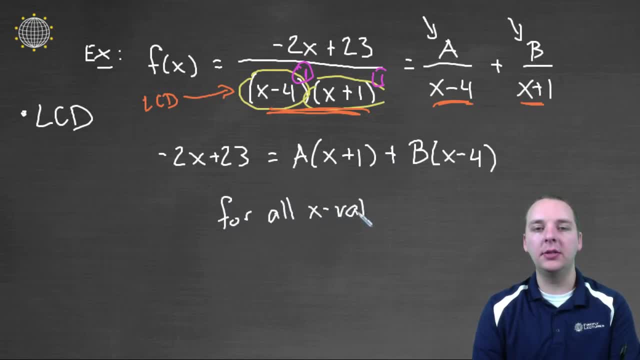 key words for all X values. right, It should be true for all X values, not some, but all X values. So what that means is we can plug in any X that we want, and this should be, should stay true. It's not true only for certain Xs. So here's what we're going to do: We're going to be smart. 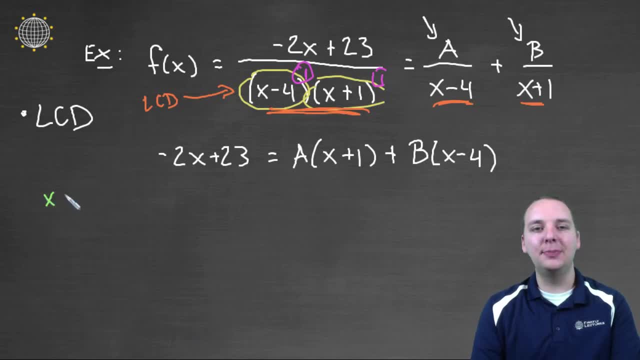 about this. This is clever. We're going to pick a specific X value, right, But we're going to pick it in a smart way. Can you think of an X value such that, when you plugged it in, it would make either the A or the B disappear? I think I can think of two. I think negative one would be a. 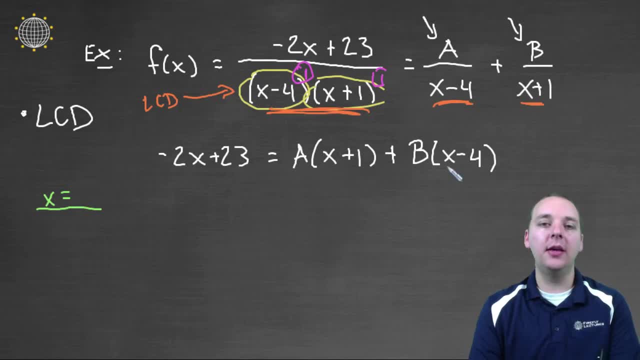 good one, because that would give you A times zero. or I think four would be a good X, because you would get B times zero. four minus four is zero, And so either one of those would be good. Let's try that. If X was negative one, let's do the math: Negative two times negative. 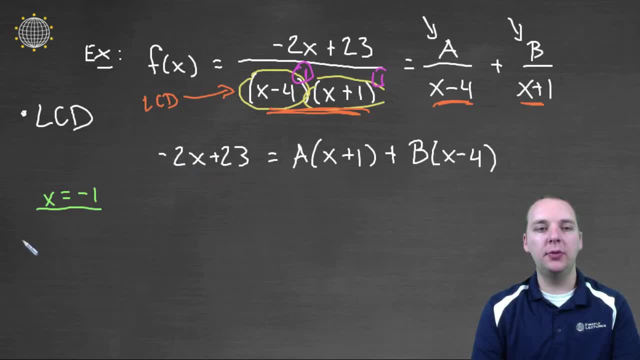 one is a positive. two, two and 23 make 25.. And this would be zero, right That, that would be gone. And negative one minus four makes negative five B. Well, you know bam, automatically, we see, B must be negative five, right? Negative five times. 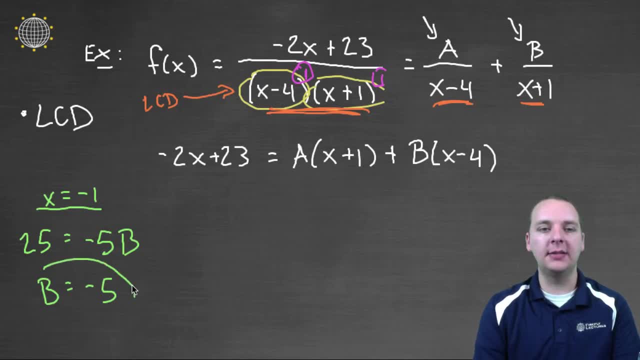 negative five is 25.. Wow, that was so. that was so nice and simple and easy. No systems, no matrices, just a nice little shortcut noticing that this was an identity. that was always true for any X. Now, let's do that other X we were talking about. X equals four. Let's do. 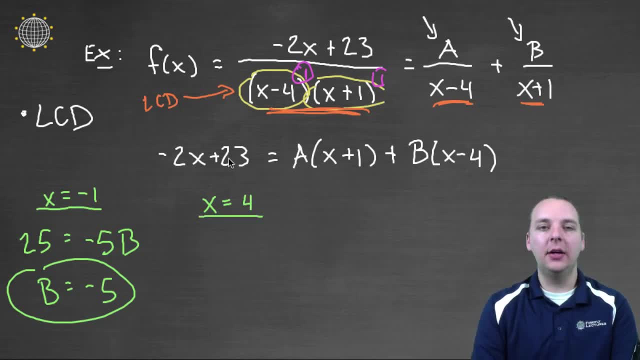 the same thing. Negative two times four is negative. eight. 23 minus eight. 23 minus eight would be 15.. And then on the right-hand side we'd have four plus one is five, So we'd have five A, five A, And so A equals 15 over five, which is three, So fast. 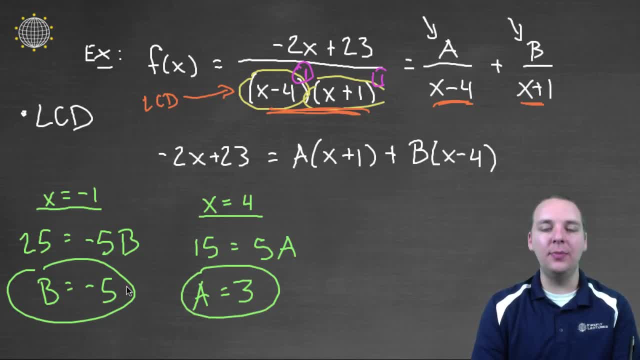 right, So quick, Uh, and that that's the A and the B, or what A and B should should be in the decomposition. So here's what we can do next. We can come up here, Um, we can erase this A and. 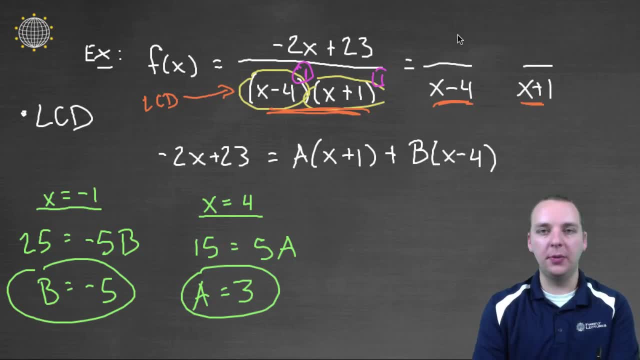 this B or you can just write a new line. You don't have to just keep erasing or whatnot. You can write a new line, but I'm just going to write it right here. Um, if this is A, then I'm going. 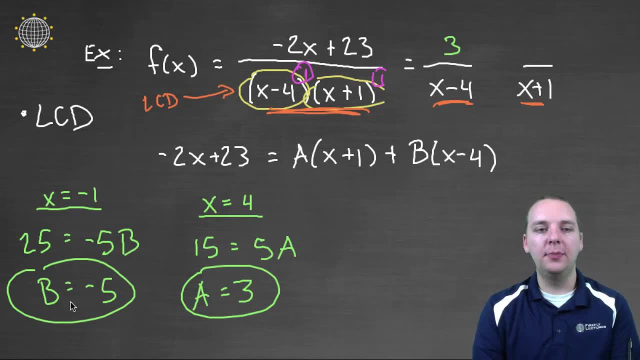 to take the A out and put a three in its place, And if B is negative five, I'll put minus five. right there, right, And we're done. That's the decomposition, That's the last step. That's how we're going to do it. So we're going to take the A out and put a three in its place, And then we're. 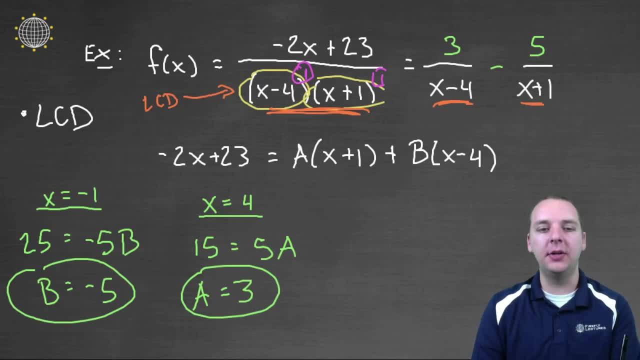 going to take the B out and put a three in its place, And then we're going to take the B out and put a three in its place, And then we're going to take the B out and put a three in its place. Now in a, in a bigger sense, what was the ultimate goal? Again, I've I've said this in most of our